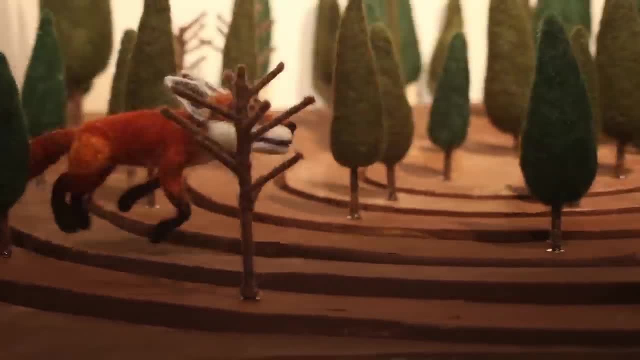 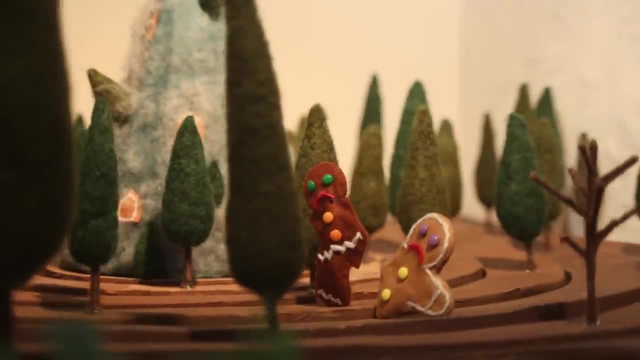 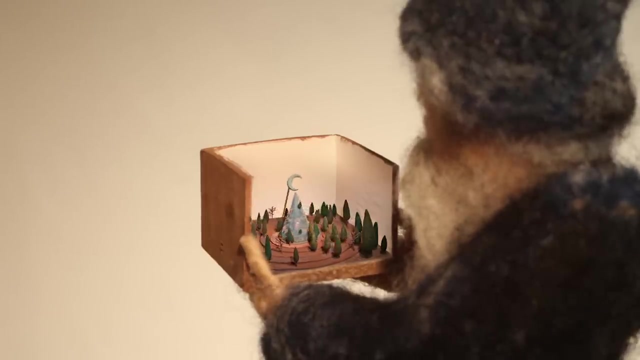 Crispy and Chewy act accordingly, and the smug fox runs off with a belly full of gingerbread, leaving the two former friends with just one leg to stand on. Normally, this is where the story would end, but a wizard happened to be watching the whole mess unfold. 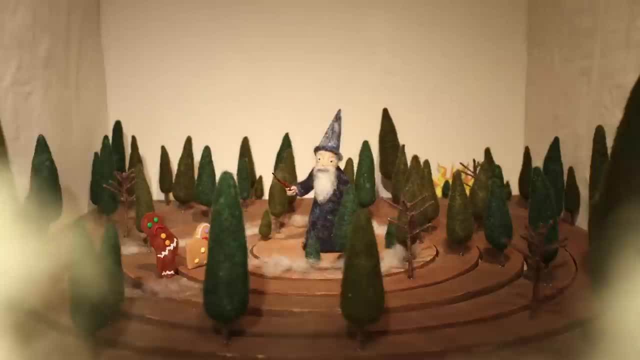 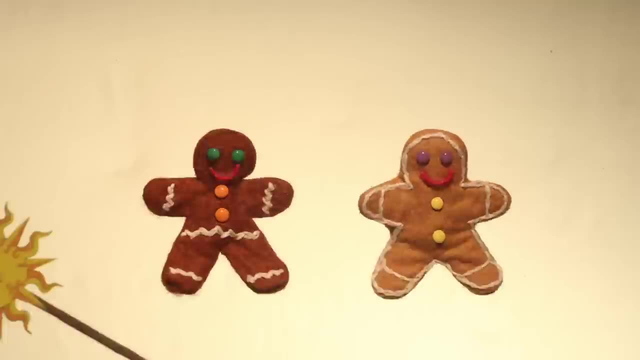 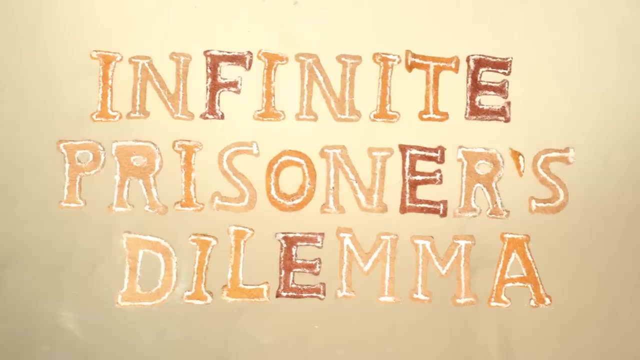 He tells Crispy and Chewy that, as punishment for betraying each other, they're doomed to repeat this dilemma for the rest of their lives, starting with all four limbs at each sunrise. Now what happens? This is called an infinite prisoner's dilemma. 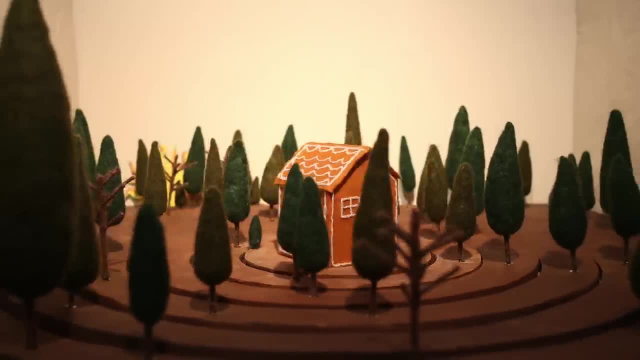 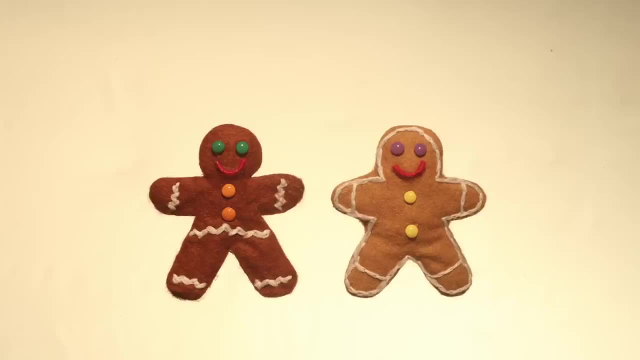 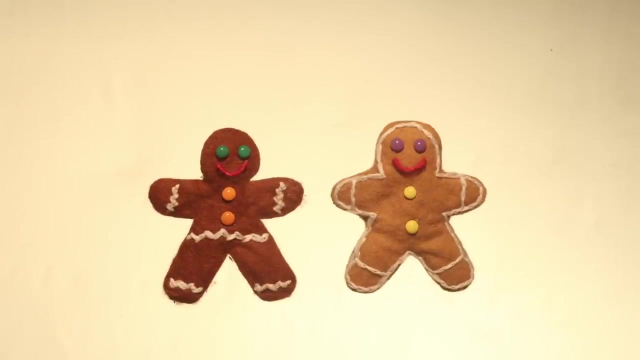 and it's a literal game changer. That's because the gingerbread men can now use their future decisions as bargaining chips for the present ones. Consider this strategy: Both agree to spare each other every day. If one ever chooses to sacrifice, the other will retaliate by choosing sacrifice for the rest of eternity. 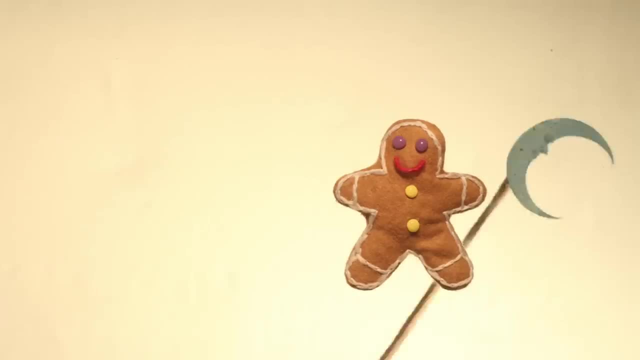 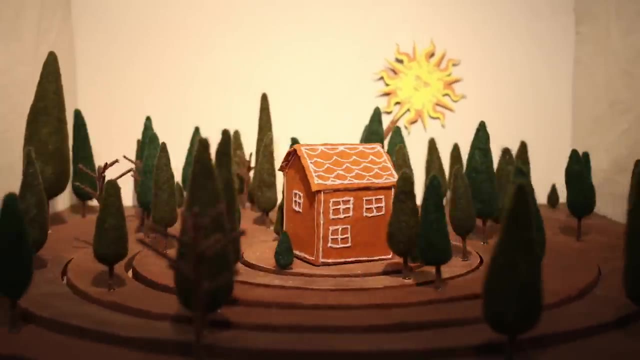 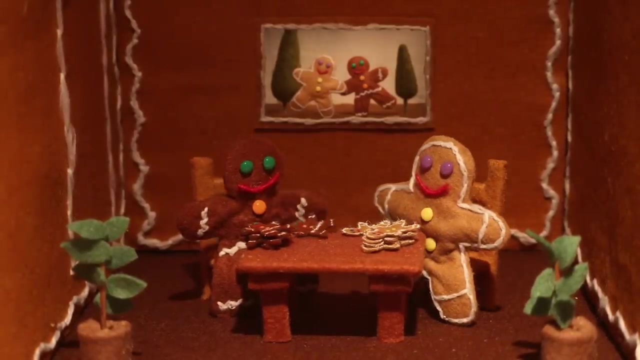 So is that enough to get these poor sentient baked goods to agree to cooperate? To figure that out we have to factor in another consideration: The gingerbread men probably care about the future less than they care about the present. In other words, they might discount how much they care about their future limbs. 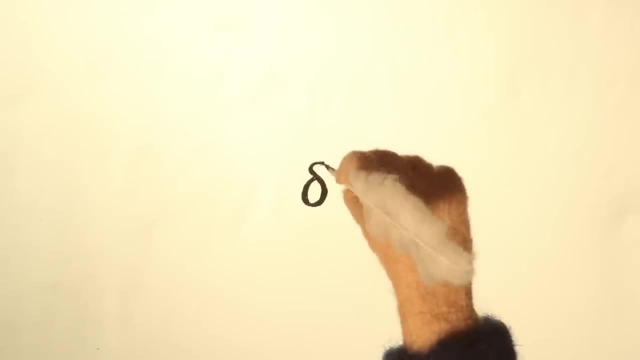 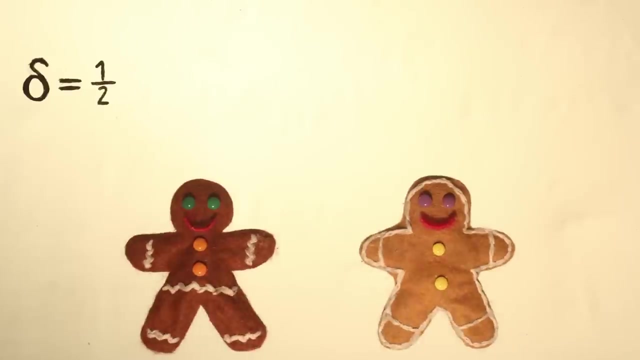 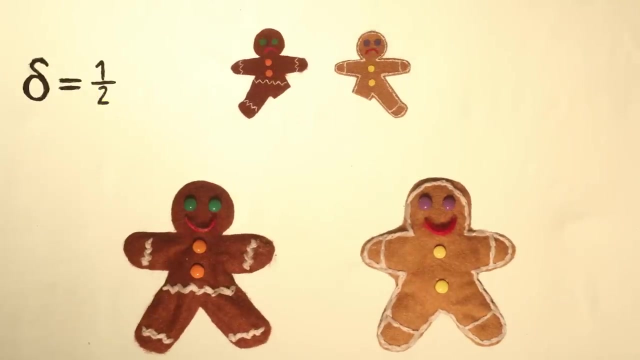 by some number, which we'll call delta. This is similar to the idea of inflation eroding the value of money. If delta is one half on day one, they care about day two limbs half as much as day one limbs. day three limbs one quarter as much as day one limbs. 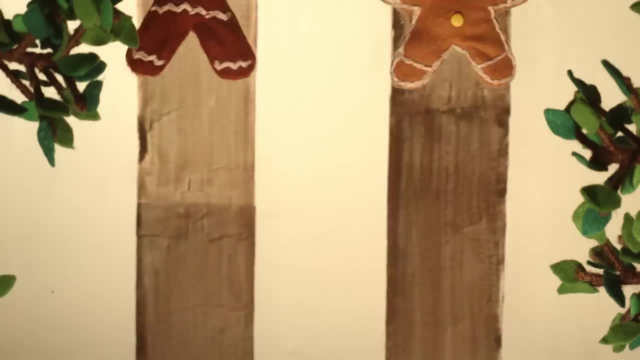 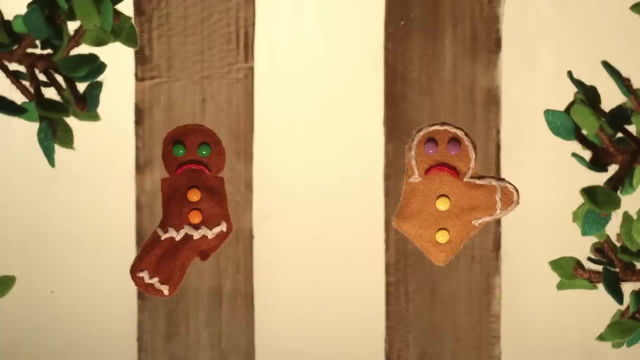 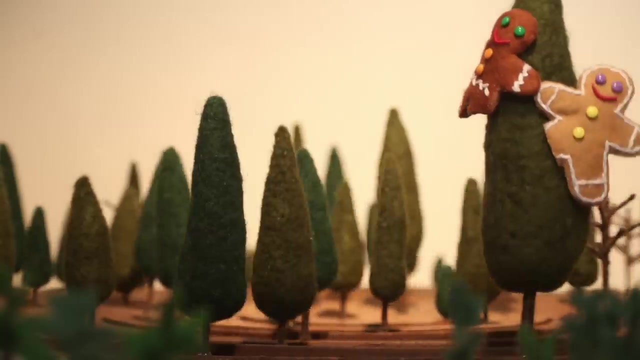 and so on. A delta of zero means that they don't care about their future limbs at all. so they'll repeat their initial choice of mutual sacrifice endlessly. But as delta approaches one, they'll do anything possible to avoid the pain of infinite triple-limb consumption. 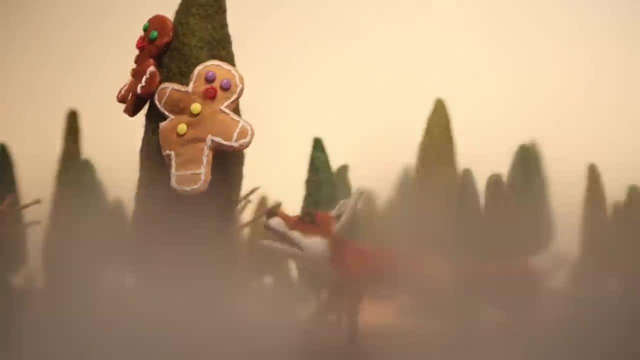 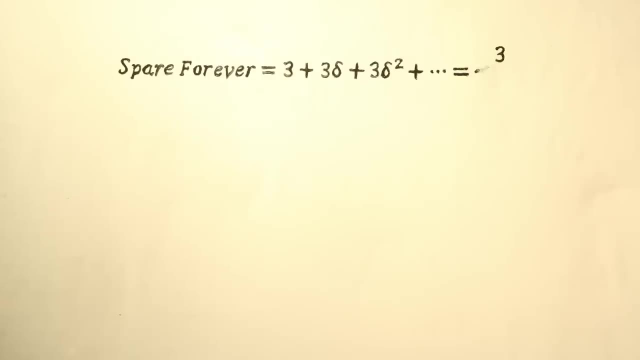 which means they'll choose to spare each other At some point in between. they could go either way. We can find out where that point is by writing the infinite series that represents the number of limbs. It represents each strategy, setting them equal to each other and solving for delta.